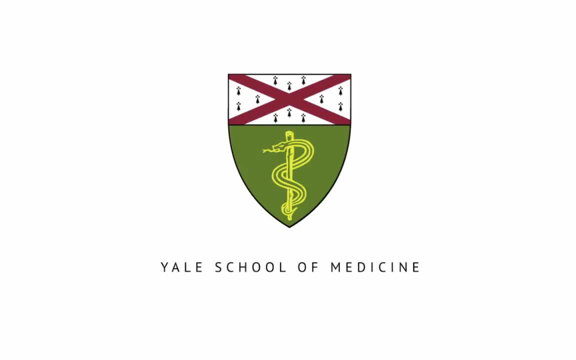 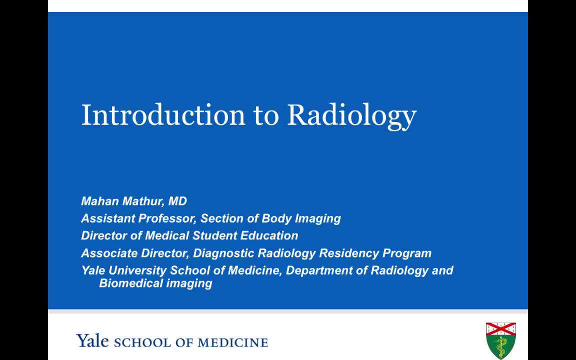 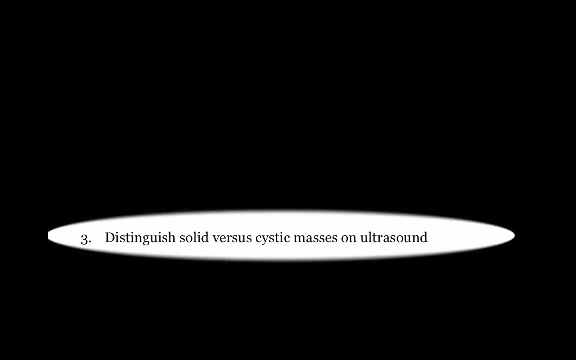 Hello, this is Mahan Mathur, and this is the third video in our lecture series on introduction to radiology. In this video, we'll cover ultrasound imaging, and the objective for this video is to be able to distinguish solid versus cystic masses on ultrasound. Like the prior videos, we'll start off with a brief. 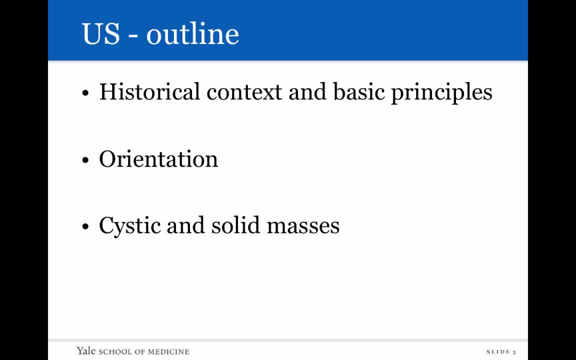 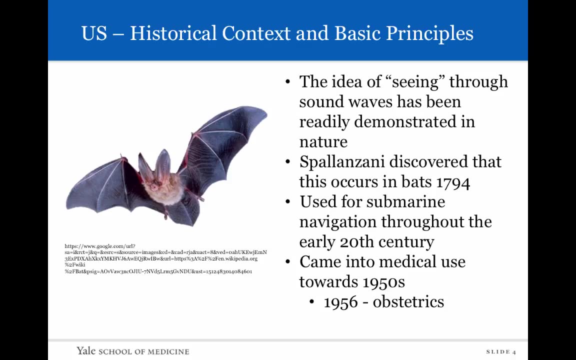 foray into the historical context of ultrasound imaging, go over some basic principles. we'll then move on to basic orientation on ultrasound imaging, followed by what cystic masses look like and what solid masses look like. So ultrasound imaging as a concept has been around for a very long time. In fact, if 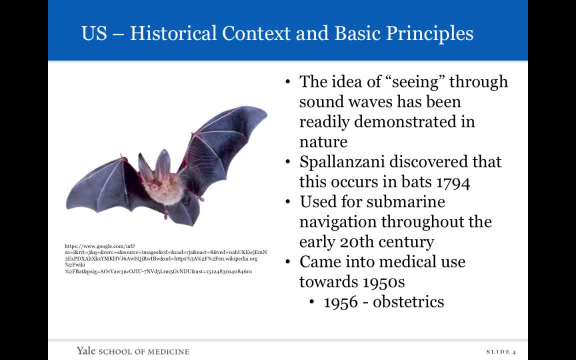 you look at bats. this idea of seeing through sound waves has been found in nature for a long time and there were some Italian scientists who discovered that this actually occurs in bats. This was back in 1794.. They actually blindfolded the bats and asked them to go from point A to point B. 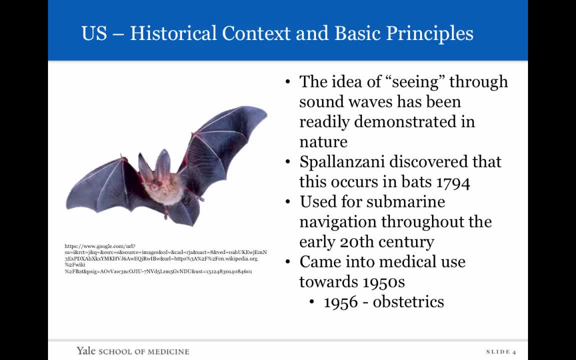 which is a food source, and they found that the bats could get there with a blindfold on. It had been used throughout the 20th century for submarine navigation and only came to the medical use around the 1950s, particularly the mid 1950s, where it was used for obstetrics. The reason that it was 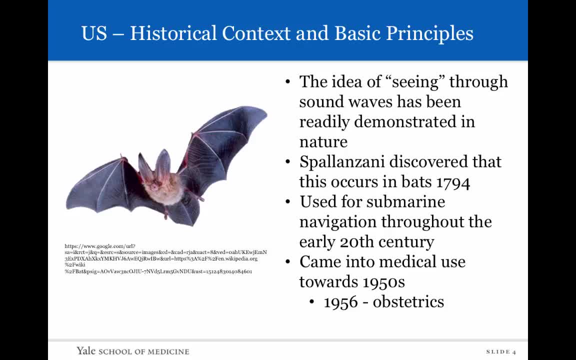 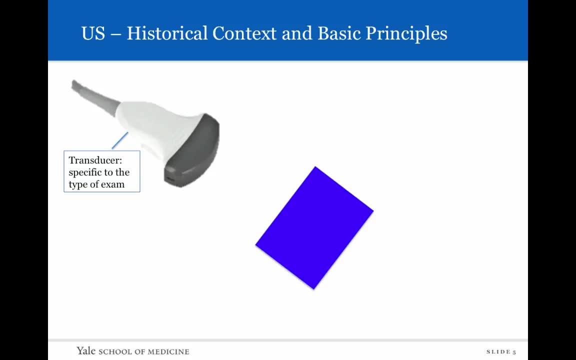 popular for use in obstetrics is because, unlike CT imaging and conventional radiography, which uses x-rays, ultrasound uses sound waves, so there's no ionizing radiation. thus, there's no risk of damage through the sound waves to the patient's body. So how does ultrasound work? Well, there's some equipment that's needed. 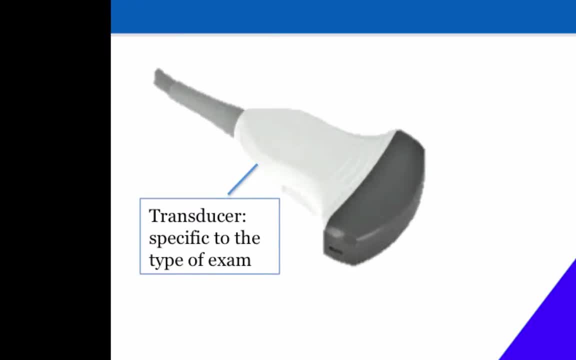 Firstly, you have a transducer, and there are several different types of transducers and they're specific to the type of exam. Some transducers will emit sound waves that allow you to penetrate deeper tissue, while some will allow you to penetrate only more superficial tissue and depending on what you want to, 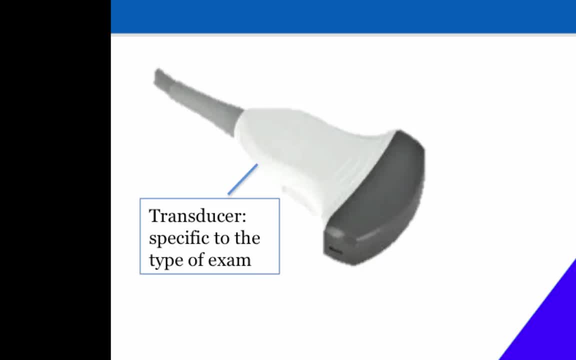 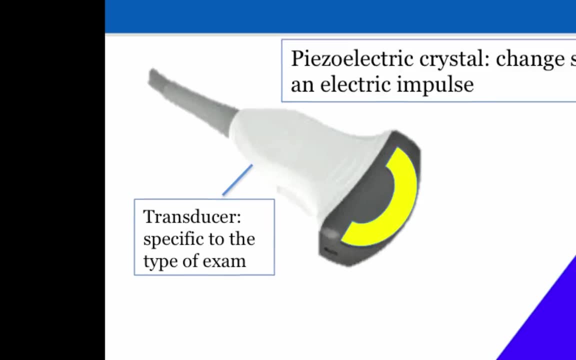 see whether it's a thyroid gland, which is superficial, or some of the abdominal organs which are a little bit deeper. you can use that appropriate transducer. Now, inside this transducer, there is a special structure that is used to connect the transducer to the transducer. So what this is is a structure made up of. 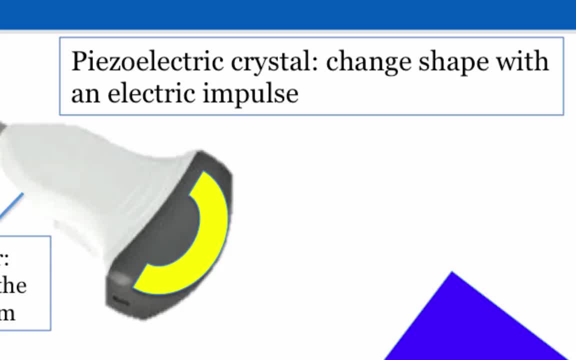 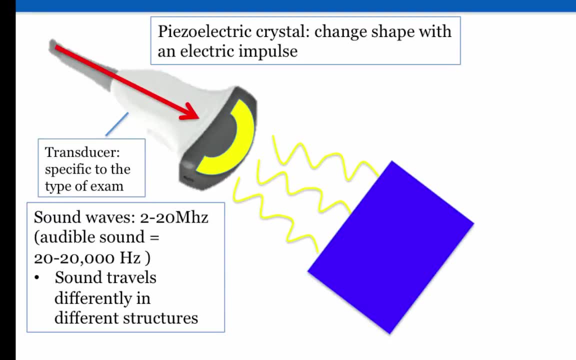 piezoelectric crystals, and what these crystals do is that they change shape with an electrical impulse. So if we give an electrical impulse, they'll start to vibrate, get bigger, smaller, bigger, smaller and this generates sound waves. Now these sound waves go from 2 to 20 megahertz in frequency. So it compares an. 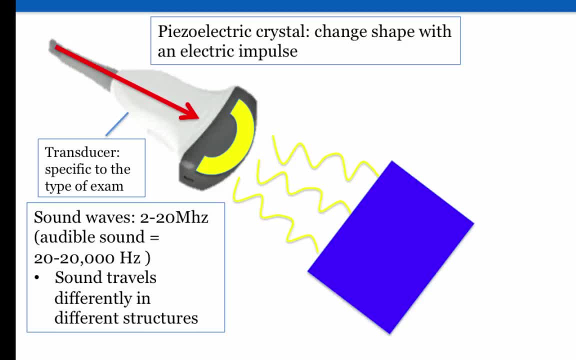 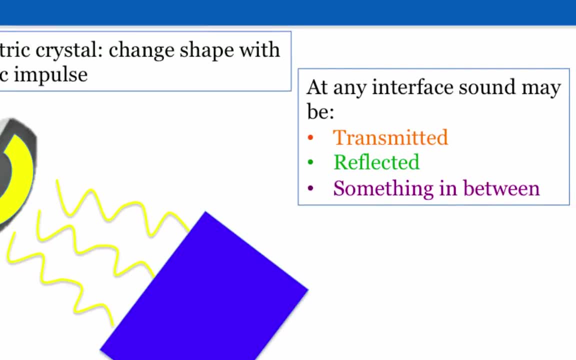 audible sound as 20 to 20,000 Hertz. so we don't hear these sound waves. and as those sound waves go through our body, they will travel differently in different structures. The sound waves may be transmitted, they may be completely reflected or often. 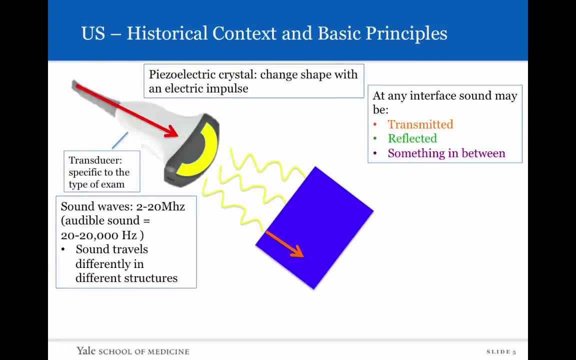 something in between, where something gets reflected, something gets transmitted, Whatever signal goes back to the transducer, this deforms this piezoelectric crystal again and that results in electrical impulse that then gets recorded by a computer. So if we were to look at an ultrasound image, 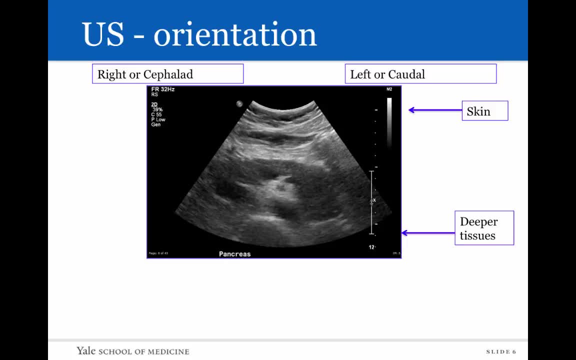 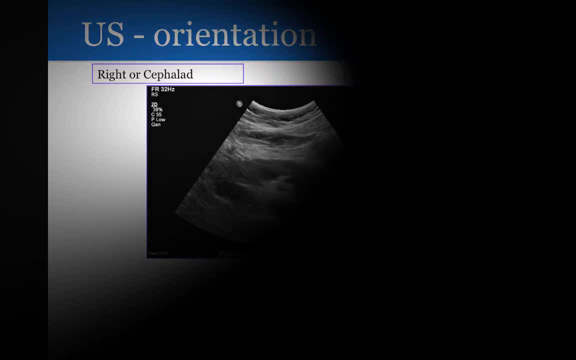 basic orientation. you can either have the probe so that you slice through the patient in an axial plane or through a sagittal plane, in which case this side of the patient will always be either the right side or cephalid, and the other side will be the left side. 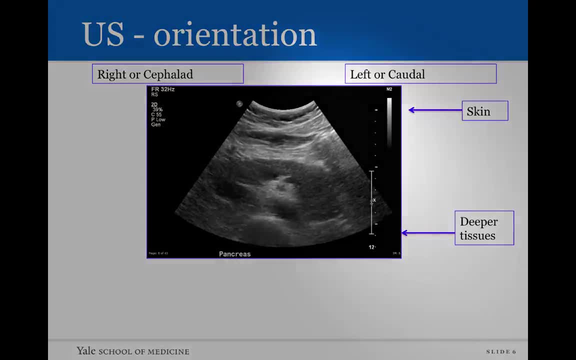 depending on whether it's an axial or a sagittal cut, Or this side of the patient will be the left side or the caudal aspect of the patient. The side over here is always the most superficial aspect, so this is going to be the skin. 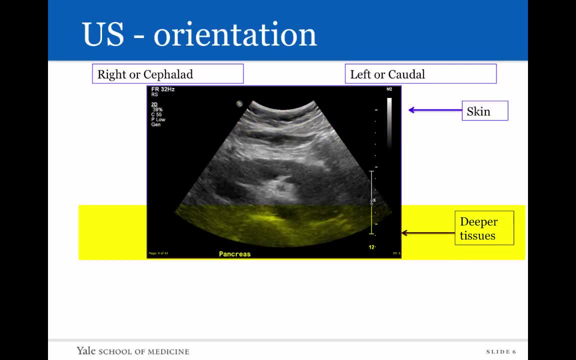 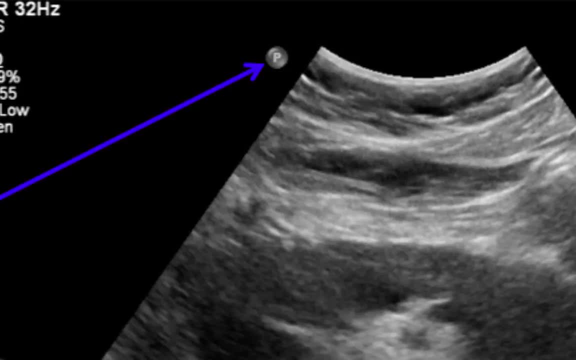 this is where the transducer will be placed, and as you go deeper, these will be the deeper tissues. on every ultrasound image there is a little marker called a probe marker. It's marked by this small letter P over here, and this can also be found on the transducer itself, where there's a little bump. 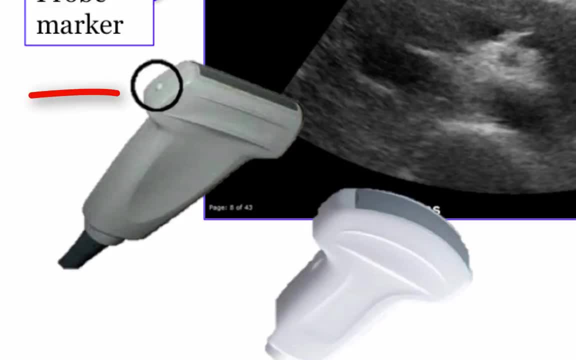 that corresponds to where that probe marker should be. It could see it over here in this linear transducer that's useful to look at more superficial structures such as the thyroid gland, and we can see it here on this curved transducer that penetrates into deeper tissues. 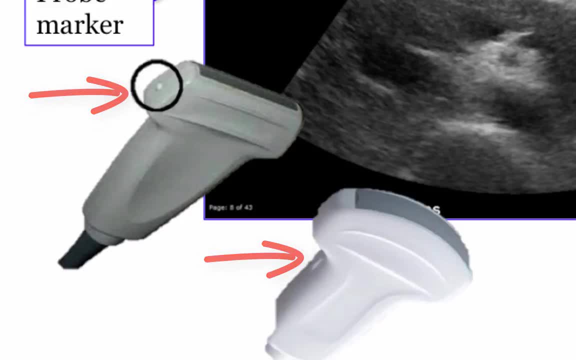 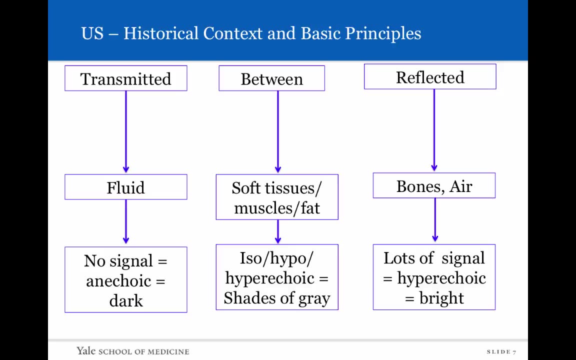 and allows us to look at structures like the liver, the pancreas, the spleen, etc. and so, if we go back to the concept of the sound waves interacting with different tissues, as we mentioned, they can be completely transmitted through that tissue, they could be completely reflected, or often something in between. now, if something's made up of pure fluid, it turns out. 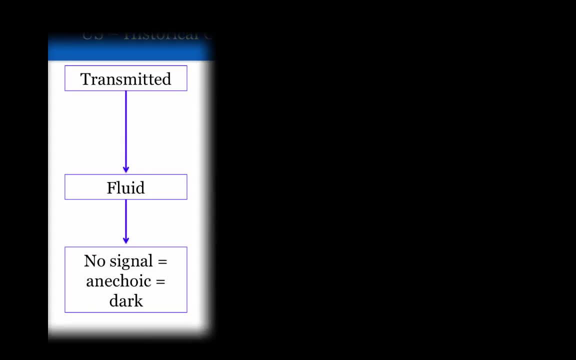 the sound waves will go directly through that fluid filled structure. as a result, there will be a positive signal that goes back to the transducer and that will appear black, anechoic, dark on imaging, as we'll see in the next few slides, if something is completely reflected. 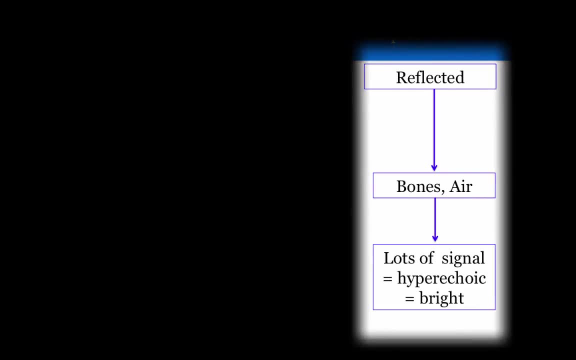 back, as can be seen with the interaction of sound with bones and air interfaces. well, there's lots of signal because everything is going to go back to the transducer, so it'll appear very bright or hyperechoic and everything behind that area will not be seen. 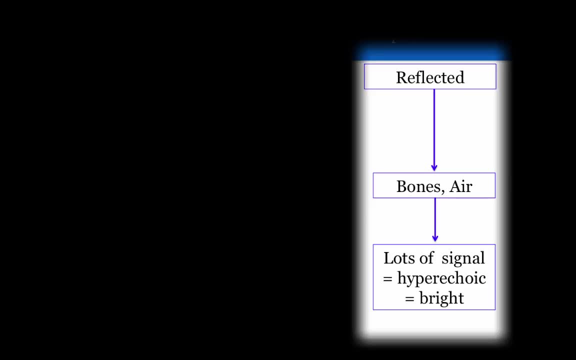 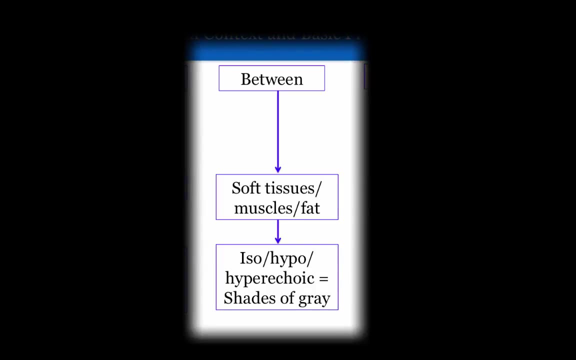 because there's nothing that's going through, so that everything behind that area that's reflect will be very dark. and if it goes in between most tissues like soft tissues, muscles and fat, well it can be either different shades of gray and it can be very bright or hyperechoic, very dark or hypoechoic, or 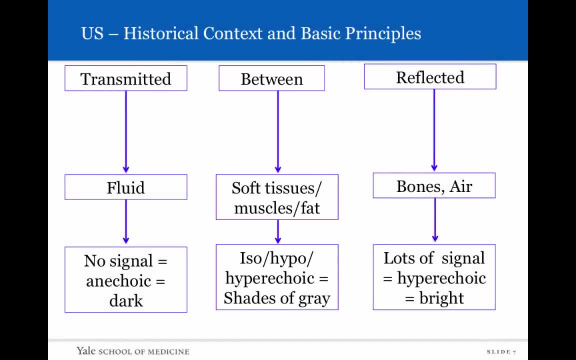 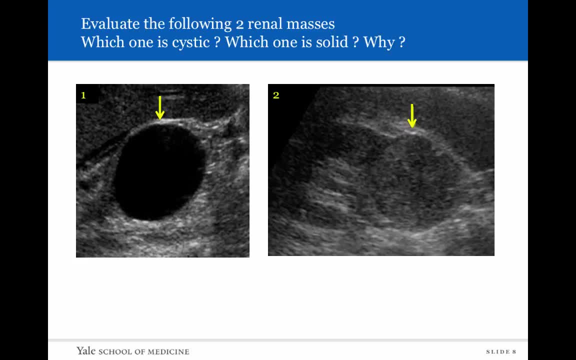 can look like the rat surrounding soft tissue, in which case we call it isoechoic. so if you use those two concepts to evaluate this case, look at these two renal masses, which one is cystic and which one is solid, and why do you think so? well as you may have guessed this, 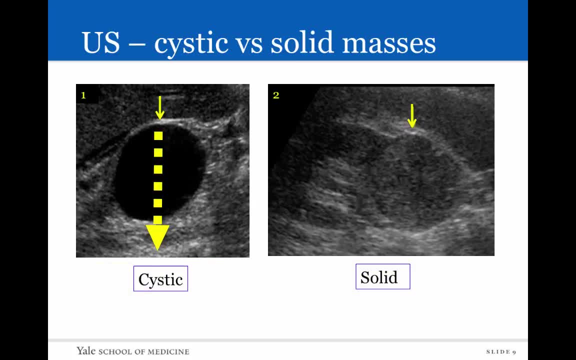 structure here is cystic, while this one is solid. as the sound waves goes through the structure, nothing gets reflected back from the structure itself, only from its interfaces or its peripheral borders. therefore, there is no signal inside this structure and therefore we know that it's something that is cystic if we look. 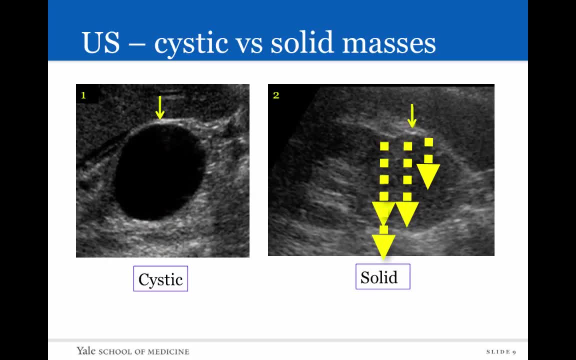 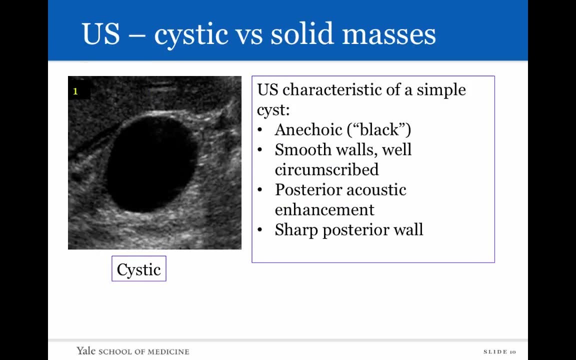 at this case over here, as the sound waves go through. some of them may pass through, but a lot of them will get also reflected backwards, resulting in a very complex appearing solid mass in this kidney. so here are some ultrasound characteristics of a simple cyst, and this applies to a cyst in any organ. 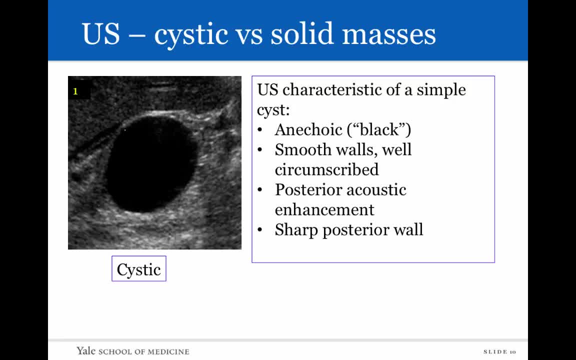 within the body. it'll be anechoic or black. the walls that we'll see will be extremely smooth, wall circumscribed. you can trace them with a pencil. the soft tissues immediately behind the cyst will actually be brighter than the adjacent soft tissues. and that's this idea of posterior acoustic enhancement, because 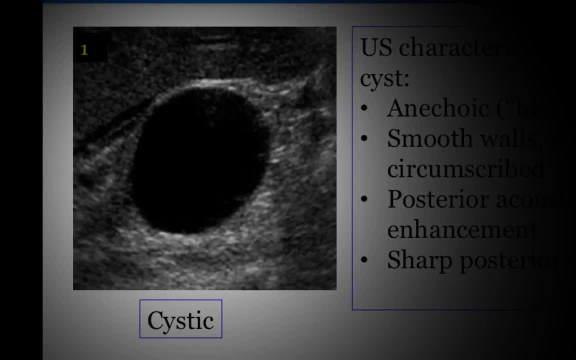 if you have sound waves going through this simple cystic structure with nothing going by, they'll go from the back side of it relatively unperturbed, as opposed to the adjacent soft tissues, where some of the sound waves will go through and some of them will go back. so